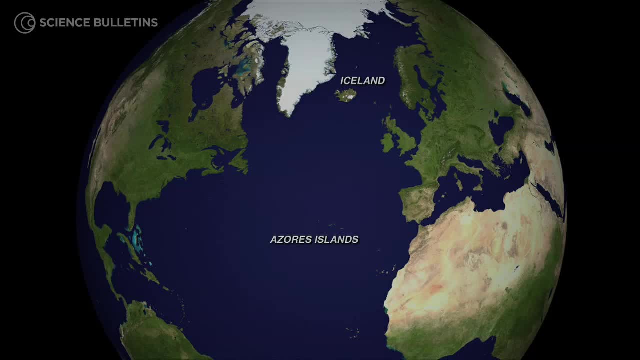 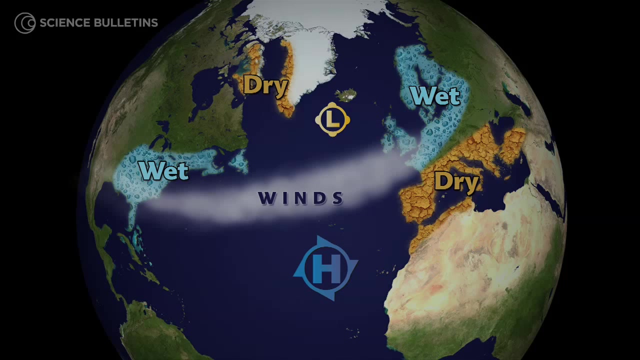 The North Atlantic Oscillation is defined by the difference in atmospheric pressure between low pressure over Iceland and high pressure over the Azore Islands, And when the pressure difference is greatest, the winds blowing from west to east across the Atlantic tend to be stronger, And this changes the distribution of temperature and precipitation from the United States through Europe and Asia. 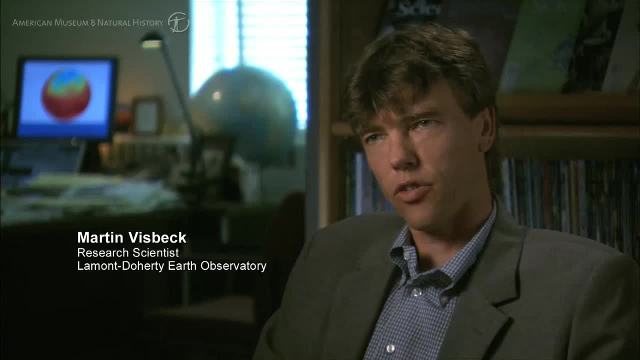 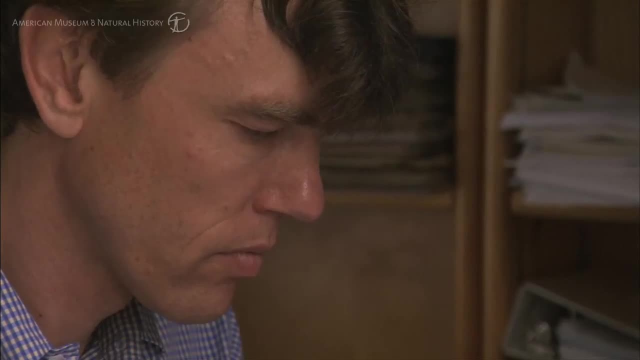 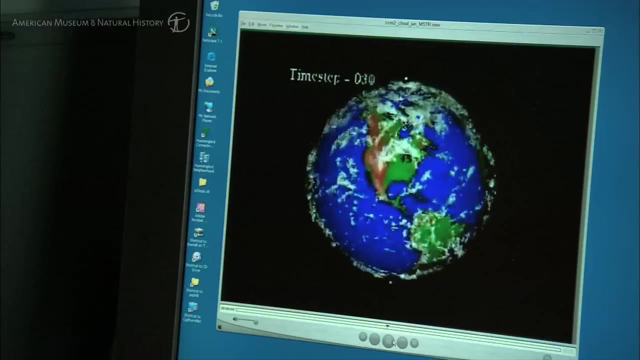 We have very well understood the basic pattern of the North Atlantic Oscillation. We have a pretty good idea about the mechanism. What we don't know yet is how to predict the North Atlantic Oscillation. The only way that we can begin to answer questions about the future behavior of the climate system is by building models of the climate system. 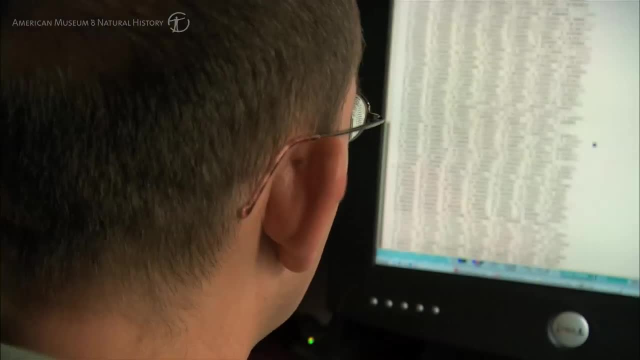 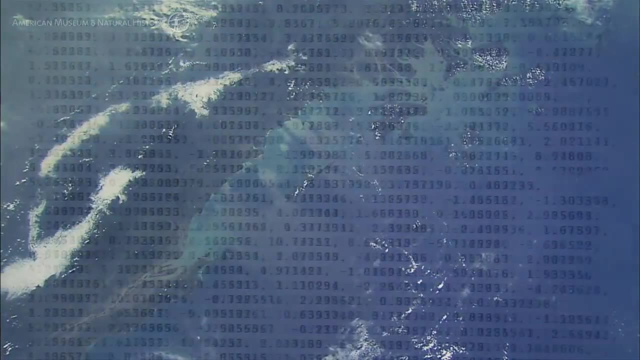 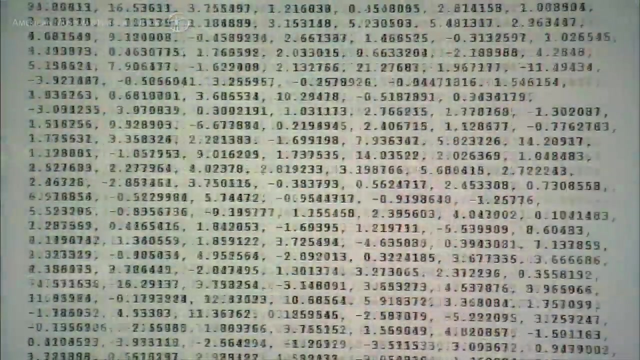 The climate model is essentially a very large set of complex mathematical equations that describe the evolution of the atmosphere, of the ocean, of the land surface. By solving this very complex set of equations, the climate model can produce its own climate that mimics how the real world operates. 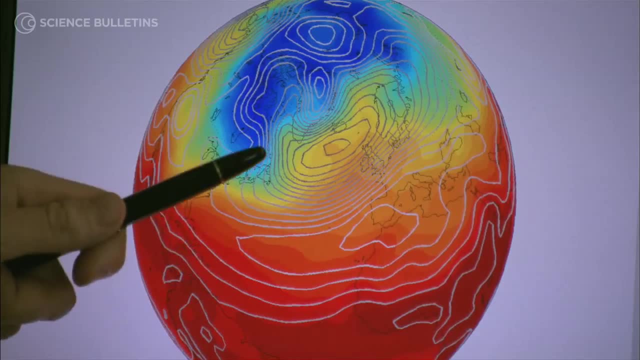 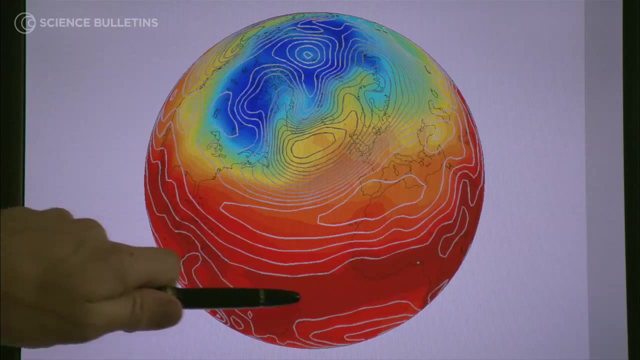 So what we see here is a snapshot of the climate condition in the North Atlantic sector. A lot of lines together mean there's very strong winds following parallel to these lines from west to east. What we study when we look at the North Atlantic Oscillation is how this picture changes over time. 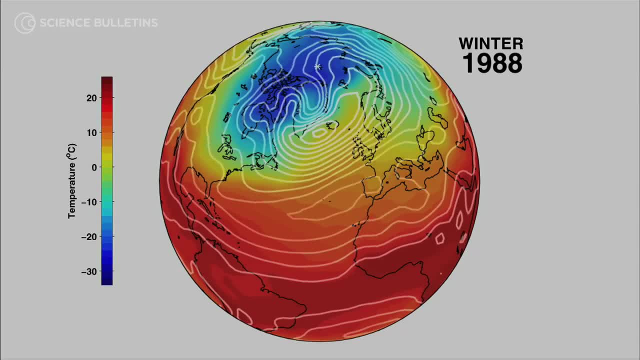 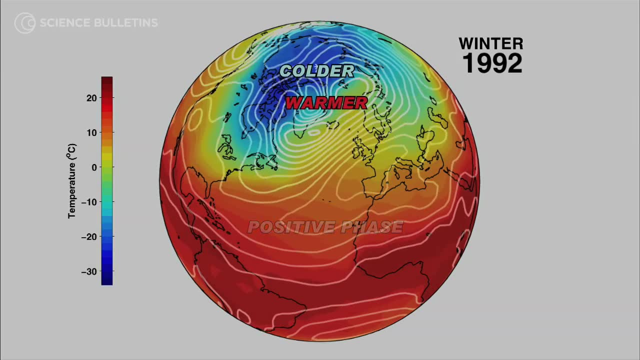 You see the temperatures in colors here And you see the cold air from the Arctic goes towards Labrador, giving you a very cold condition in northern Canada and Greenland. That would be the positive phase of the North Atlantic Oscillation. And then other times you see the cold air showing up over Europe. 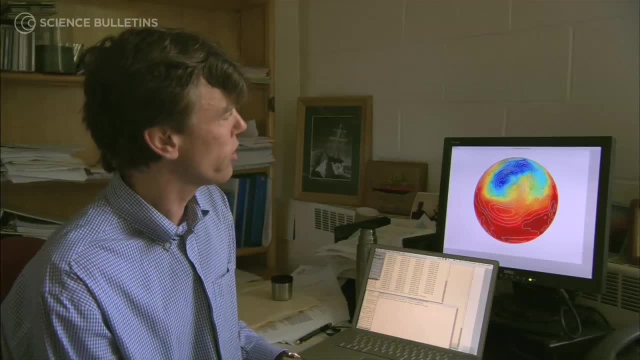 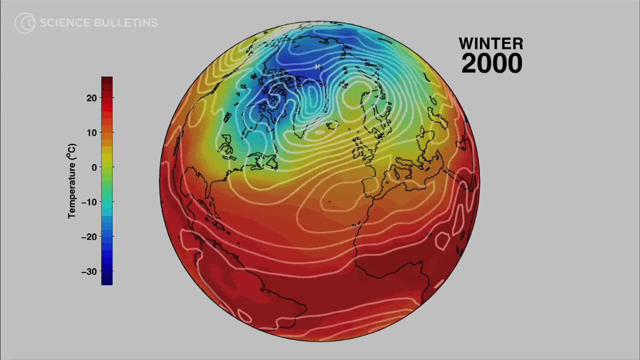 That's the negative phase of the North Atlantic Oscillation, But you've definitely noticed that it never happens at the same time. Either Europe is warm and it's very cold over Labrador, or the other way around, And this seesaw in temperatures is associated with the North Atlantic Oscillation. 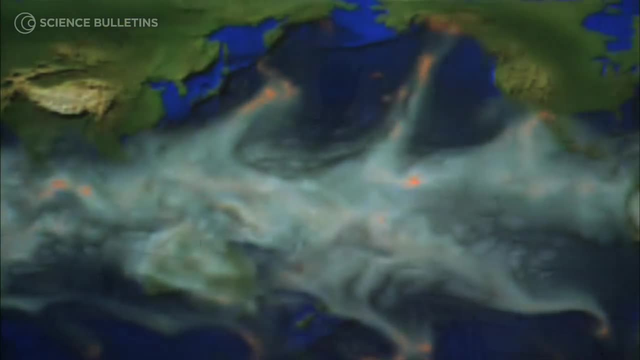 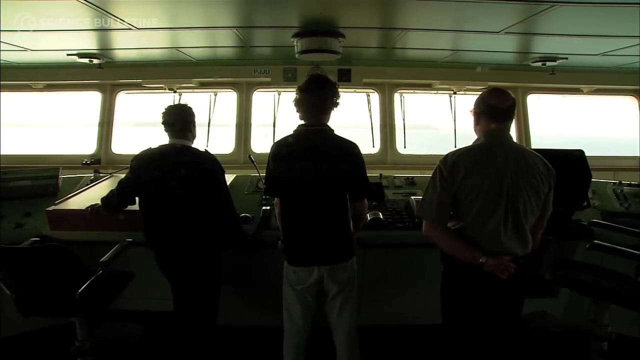 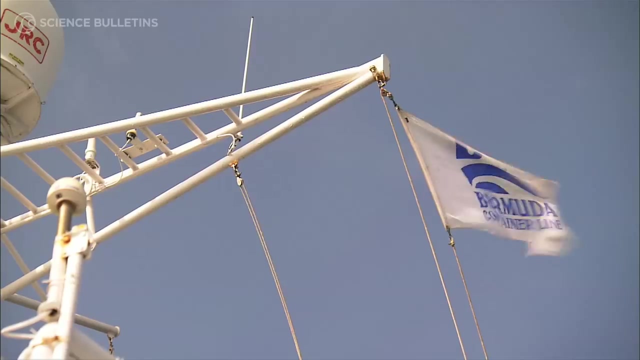 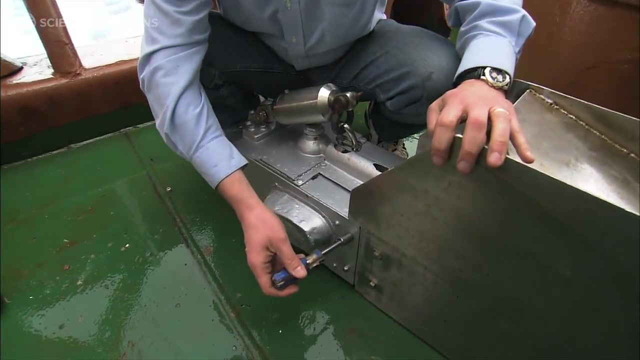 It's very important that we evaluate these models relative to reality, So we need observations of the real world. The oleander goes out into the North Atlantic Ocean and it measures the temperature, the salinity, the phytoplankton distribution, And this gives us a body of observations from which we can actually evaluate our models. 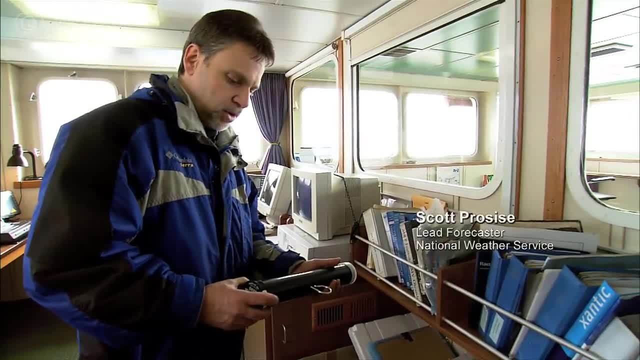 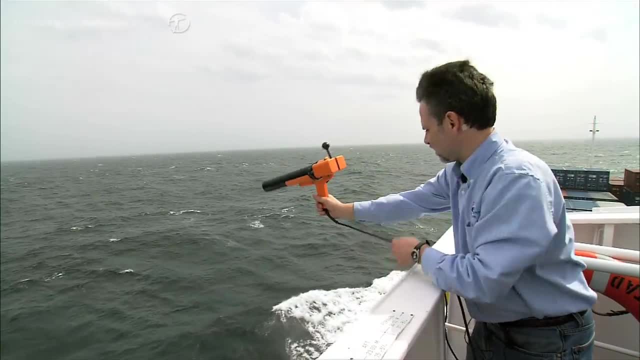 This is called a deep blue. It's a buoy that will measure the water temperature down to a depth of 750 meters. It will also continue the climatological data that the oleander has been doing for many years in logging the ocean's temperature. 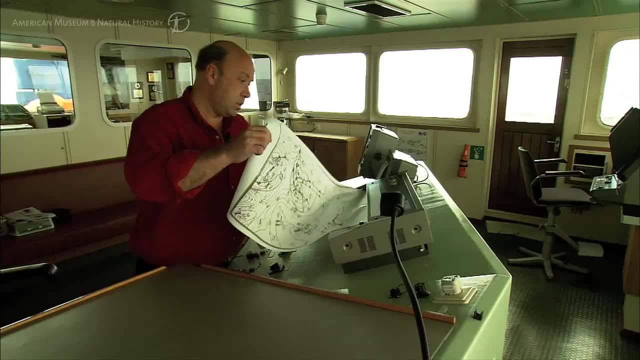 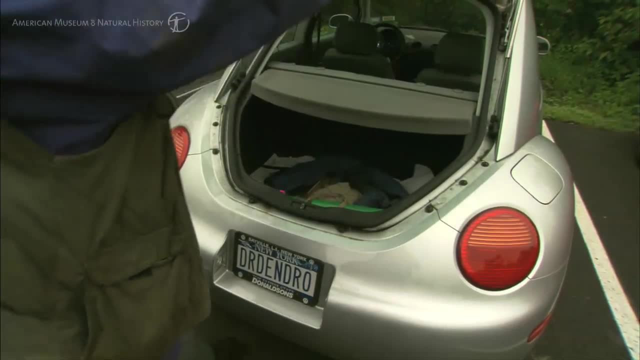 From instruments, we have about 100 years of data. What we would really like to have is a record which is 1,000 years long Now. obviously, we cannot go back and take barometric measurements 1,000 years ago, so we have to use different tools. 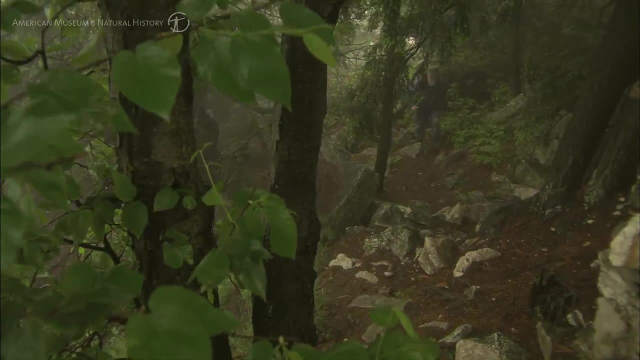 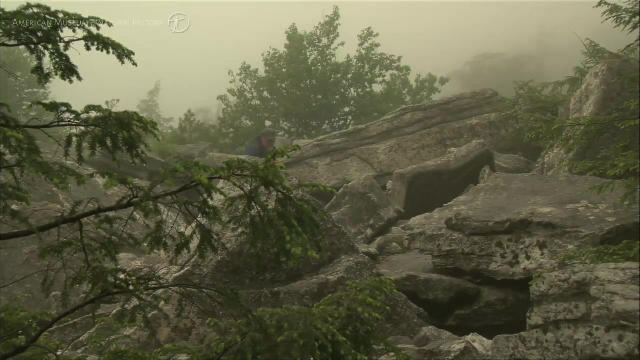 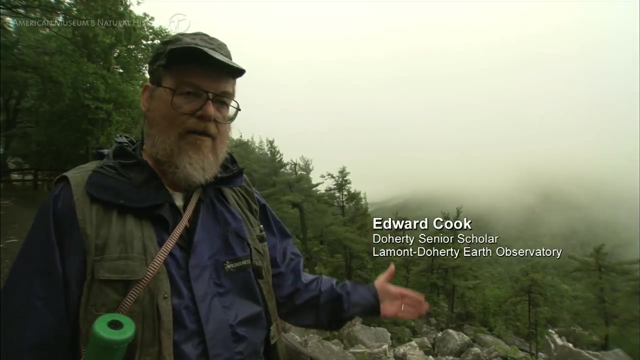 The tree research is so exciting because it's sort of a new discovery around every corner. Finding trees that are 300 or even 400 years of age is a remarkably useful discovery because we can now use the ring with variations to tell us about periods of past drought and wetness and such like that. 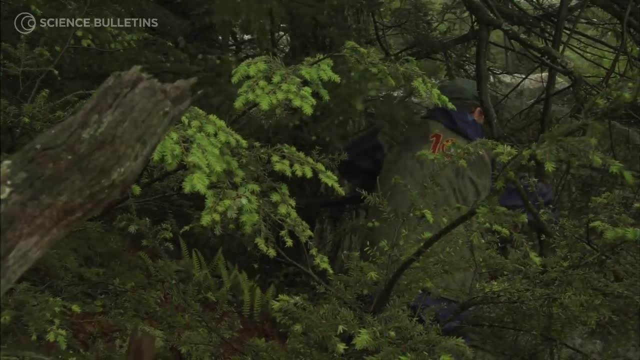 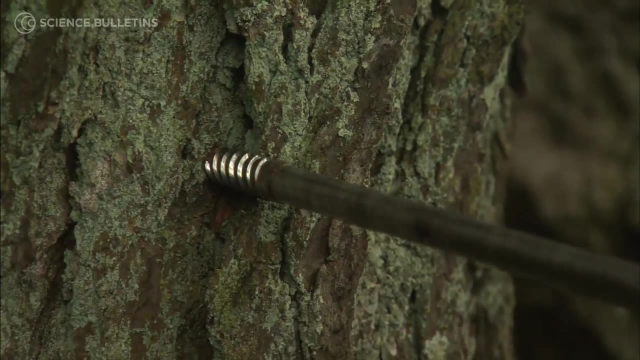 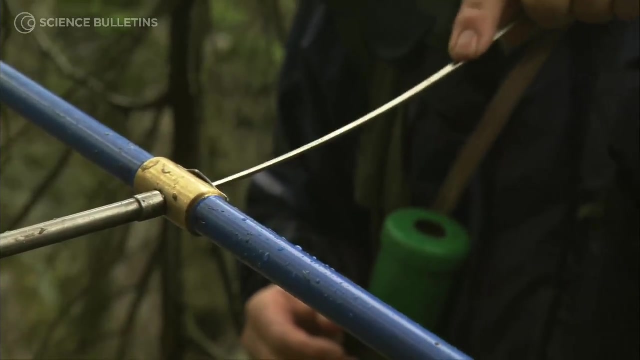 Kind of like what we're seeing right here. with the ring, We extract a 5 millimeter diameter core of wood from the tree. It's analogous to almost like a hypodermic needle for a human. This is what we would take home to the lab for analysis. 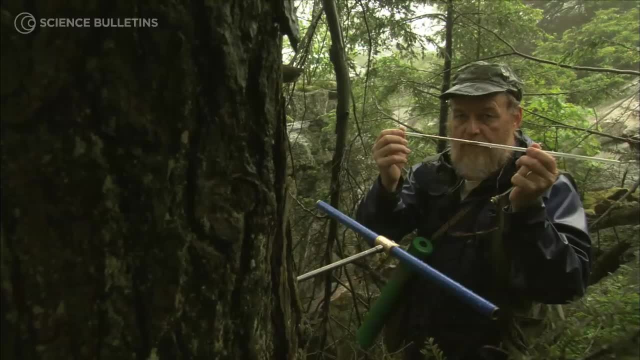 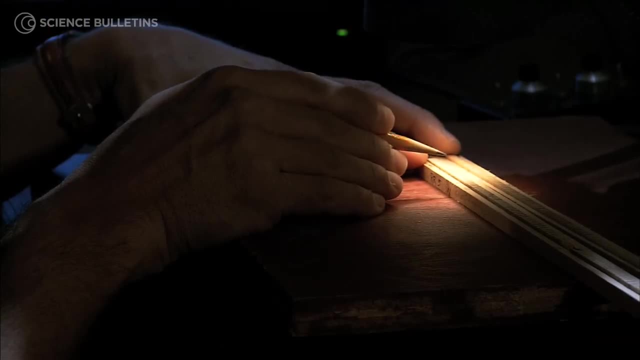 I can very clearly see the annual banding that represents each year of growth of this tree's growth. A narrow ring would mean drier than normal and a wide ring would mean wetter than normal, And all this information can be utilized to reconstruct past climate of various kinds. 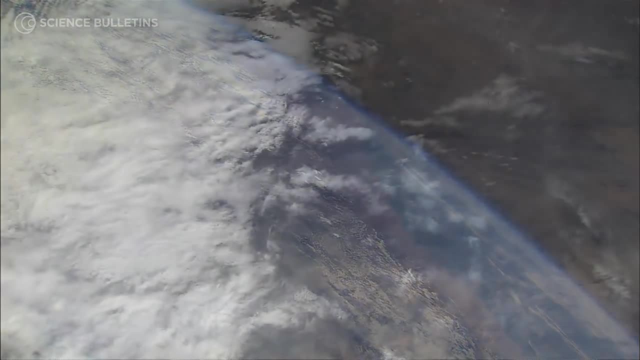 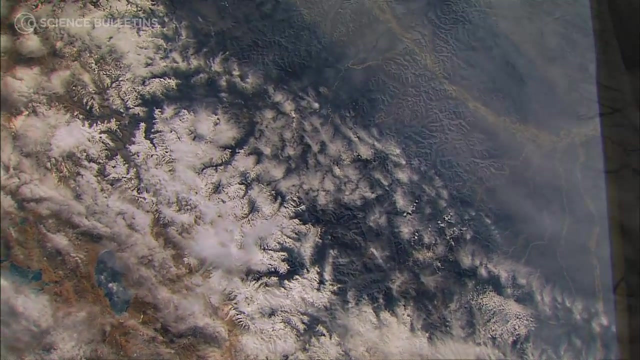 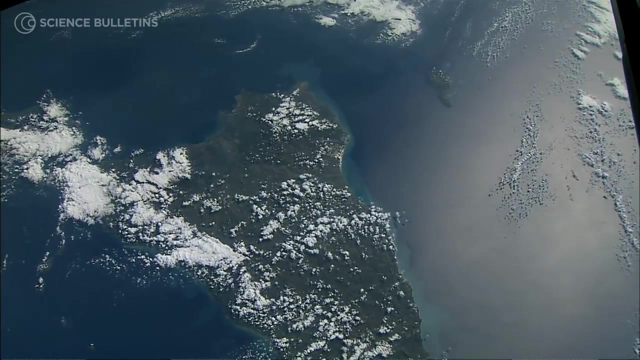 One of the factors that has really caused there to be a resurgence of interest in the North Atlantic Oscillation is: how will global warming interact with these dominant patterns of climate variability such as the North Atlantic Oscillation? So one of the key things that we need to understand is how the North Atlantic Oscillation has varied through time.